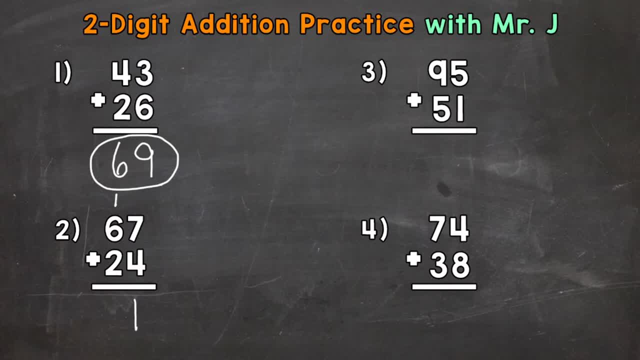 So one plus six is seven plus two is nine. Our final answer is 91.. Let's move on to number three, where we have 95 plus 51. So we'll start with the ones. Five ones plus one one equals six ones. 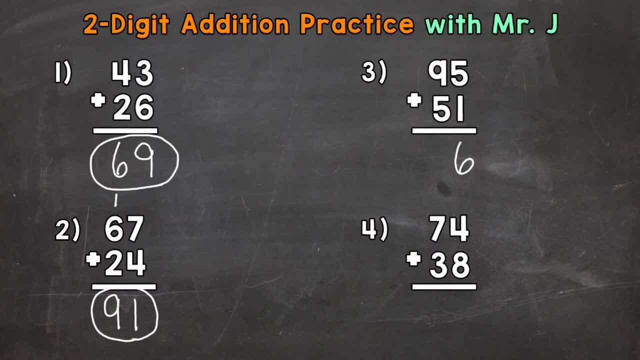 We'll move to the tens. Nine tens plus five tens equals fourteen tens. So we put the four in the tens place And regroup the one over in the hundreds, And now we can drop that one down to the hundreds place in our answer, because we don't. 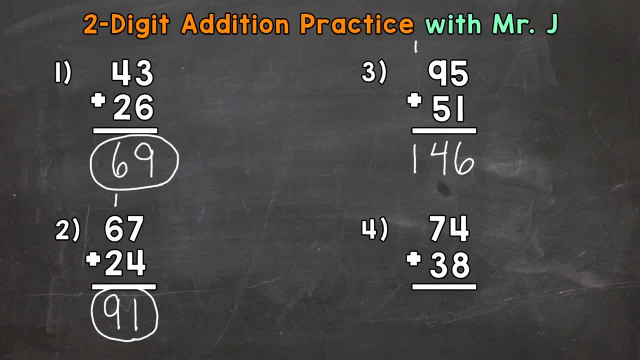 have anything else in the hundreds place. So technically it's like one plus zero plus zero, which just gives us that one. So we can think of it as just dropping that one down And our final answer is 146.. And lastly, number four: 74 plus 38.. 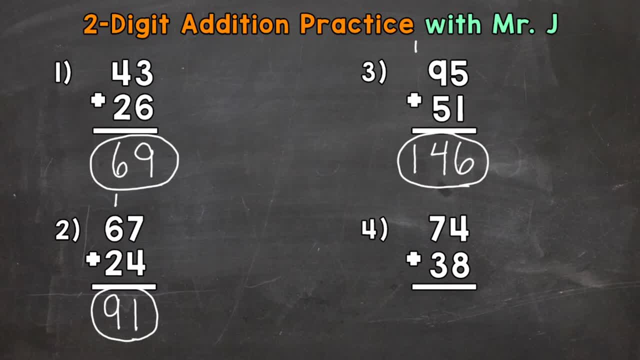 Start with the ones. Four plus eight is twelve, So we'll put our two in the ones place from twelve and then regroup the one group of ten. Now we add our tens, So one ten plus seven, tens plus three tens. 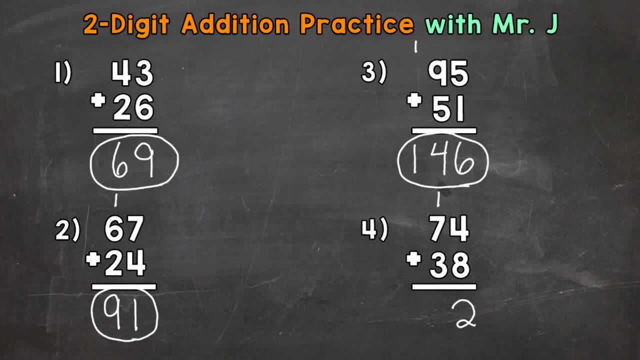 So one plus seven is eight, plus three is eleven. So we put the one in the tens place and then regroup the other one And we can bring that one down to the hundreds place, To the hundreds place in our answer And our final answer: one hundred twelve. 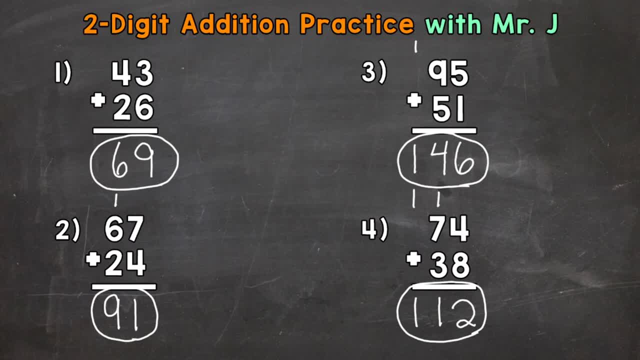 So there you have it. There are some practice problems involving two digit addition. Now, if you're looking for more addition practice or more addition help, I'll drop all of the links to my addition videos down in the description. I hope that helped. 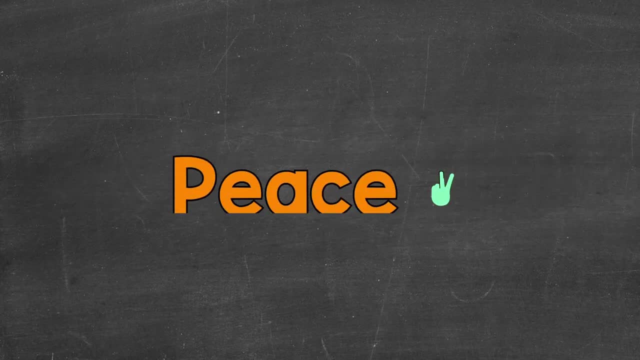 Thanks so much for watching. Until next time, peace.